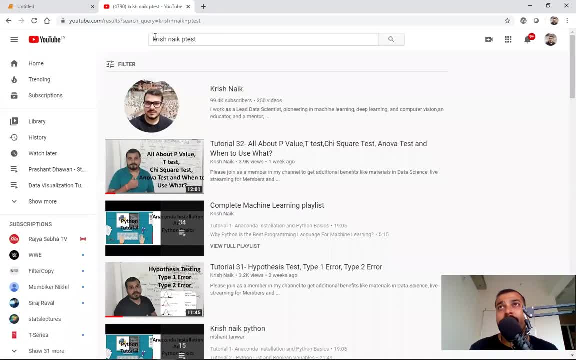 And, guys, if you don't, if you remember right in my previous video, if you just search for Krishnayak t-test or test type by test, something like that, I had actually created some theoretical video regarding it. 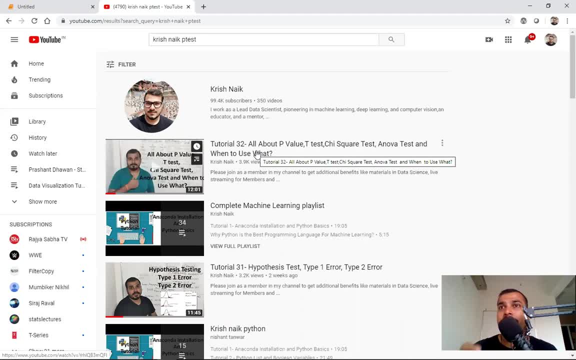 And many of you had actually requested me to implement some practical implementation with respect to Python. So in this particular video, all these particular topics, you know, we'll try to cover with the help of Python And just understand guys. in this particular video, we'll focus on understanding t-value. 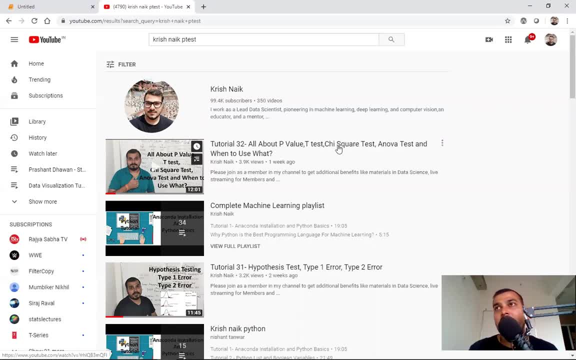 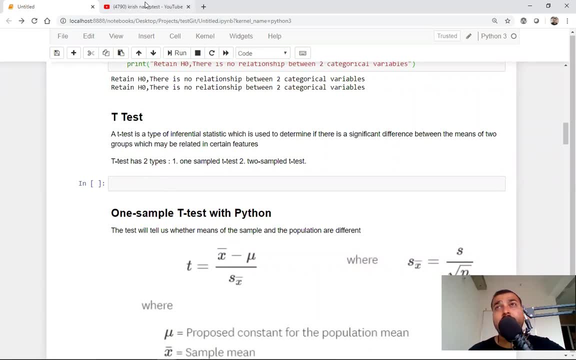 t-test and correlation. In my next upcoming video, I'll be discussing about chi-square test and I know what test. okay, So here it is. And again, guys, I would like to say that please go through this video first. Okay, if you don't understand the theoretical concept. 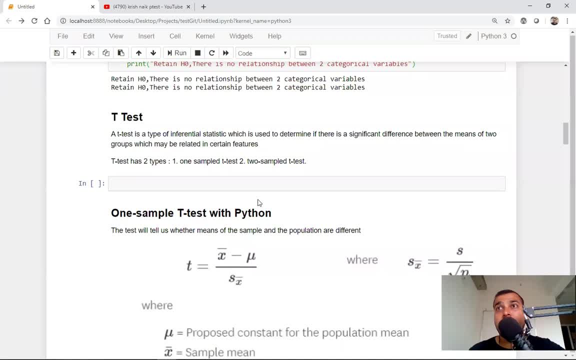 if you are able to understand the theoretical concept, then only you'll be able to understand the practical concept itself. So what is exactly a t-test? Now, t-test basically says that it is an inferential statistics which is used to determine if there is a significant difference between the means of two groups. 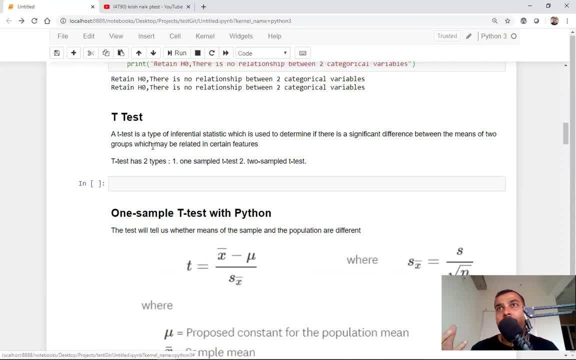 Suppose I have two groups guys and if I really want to and this two groups right, it may be a population okay, it may be a whole big population. Now, if I take the sample of two population okay and if I try to compare the mean, 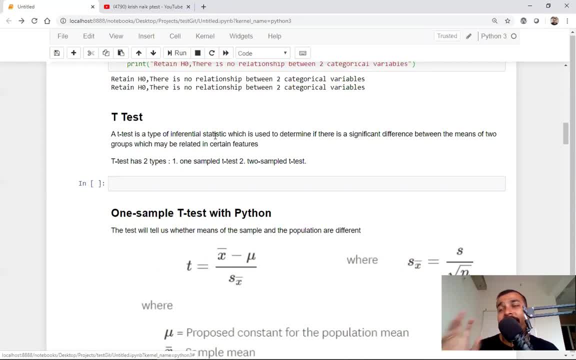 can I come to a conclusion Saying that whether there is a sound statistical difference or significant difference between this two population itself by just considering the mean from that particular population? Now I hope you have just got some idea about it. But again, understand guys. t-test usually has two types. 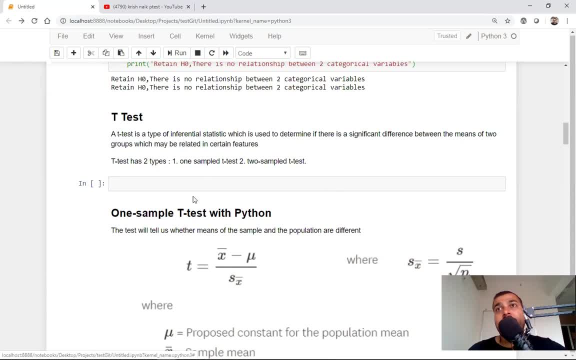 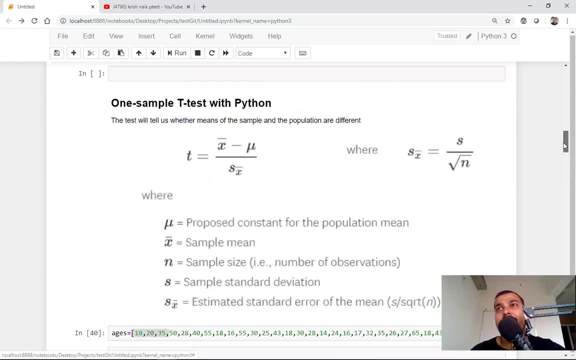 One is one sample t-test and two sample t-test. In one sample t-test. this test tells us whether means of the sample and the population are different. Now suppose, guys, I have one group, okay, and I'll show you an example what, how exactly it is done. But just understand that this is the formula. 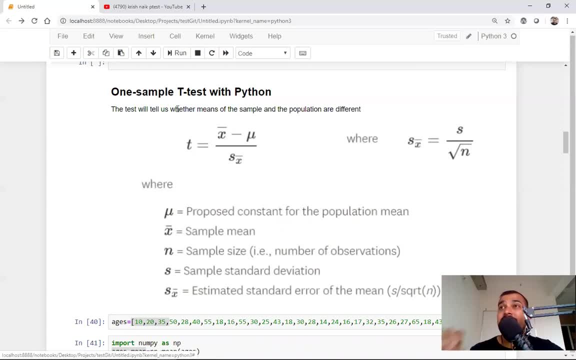 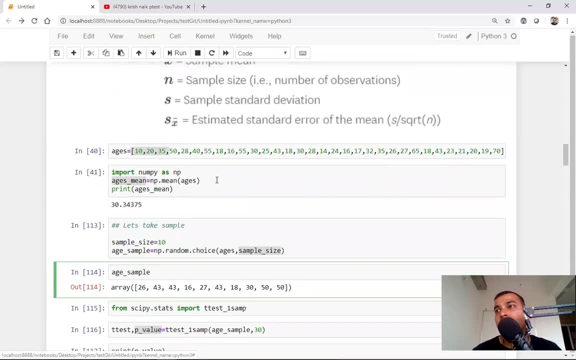 Again, the test will tell us where the mean of the sample and the population are different. okay, Now let me just consider one example with respect to one sample, with the help of Python. Now I am going to consider a class of students and I have this many people who are there. 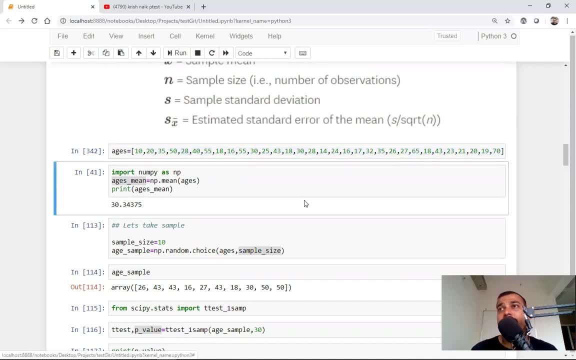 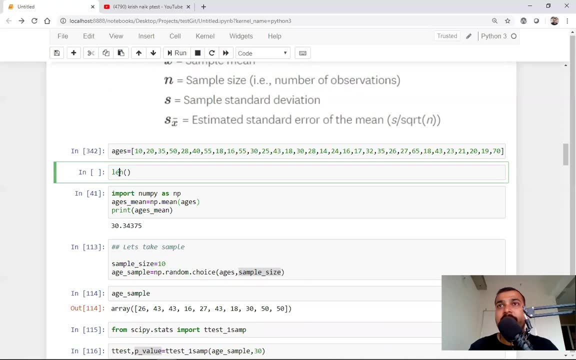 So if I just go and see how many people are there, okay, I'll just go and execute this length of ages. So I'll just let me write it as length of ages. So I'm just considering that total number of people, a total number of students are 32.. 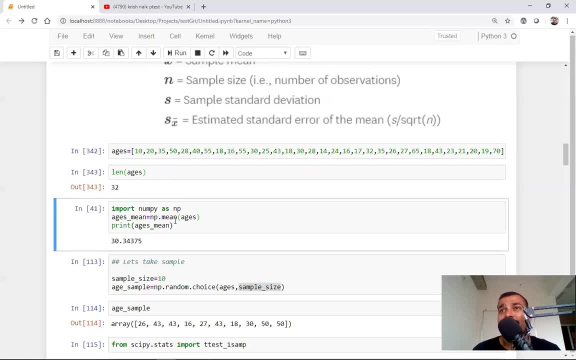 Now, if I go and calculate the mean of this, okay, so here I've imported numpy npmean of ages, So I'm getting this particular value, the mean of this particular classroom students of with respect to the age, And this may be university students. okay, guys. 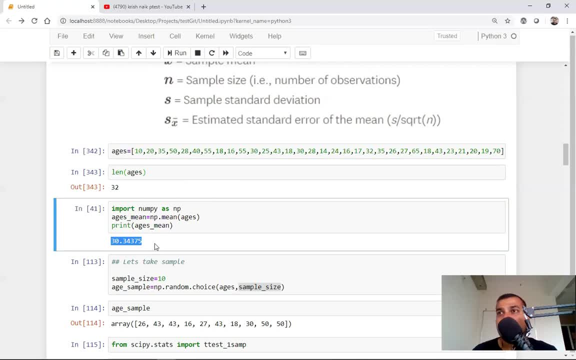 So it is somewhere around 30.34375.. Now, if I consider a sample of ages from this and if I compute a mean, is there any some significant difference between the mean of the population and the sample? That is what we want to see, okay. 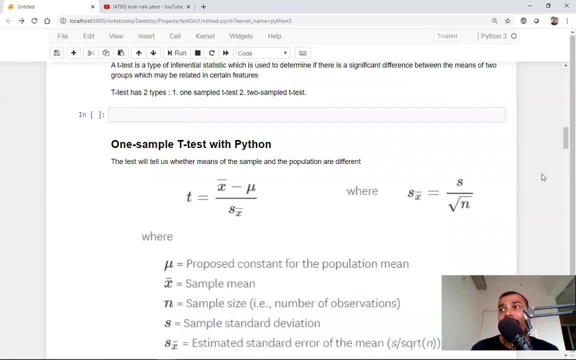 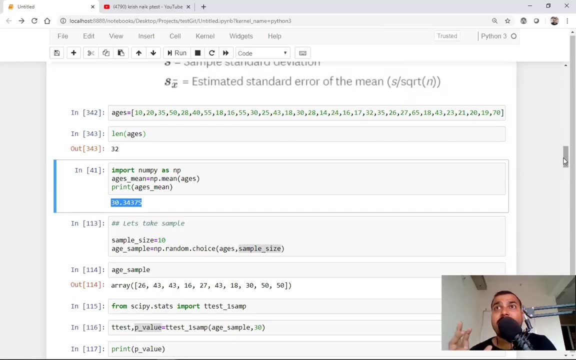 Now that can be actually done with the help of one sample t-test. And again, remember, guys, if I consider this particular problem statement and my previous video also, I've discussed that if you are doing with respect to t-test, you're basically comparing a population and the sample. 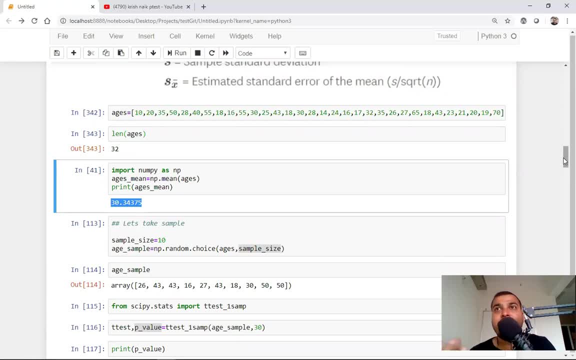 and then you are validating something based on the evidences. right Now, in this particular case, my validation is that whether there is some difference between the sample mean and the population mean. So here I'll be creating an alternate hypothesis. 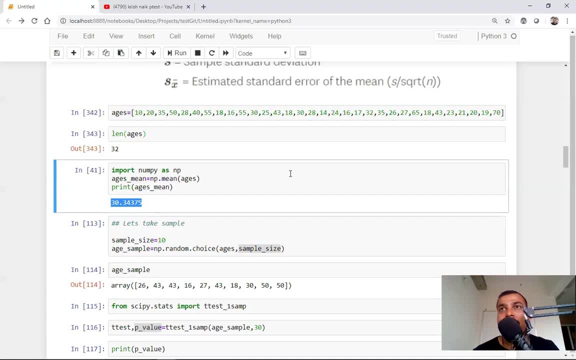 Now alternate hypothesis will say that there is a difference, okay, And my null hypothesis will say that there is no difference, okay. So again I'm repeating guys: my null hypothesis will say that there is no difference. My alternate hypothesis will say that there is a difference. 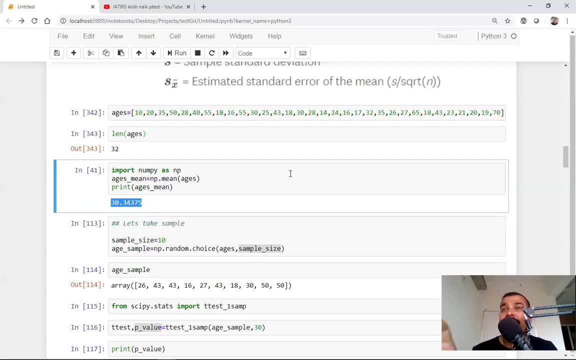 Now I'll use this one sample t-test to basically compute a p-value, And if the p-value is less than 0.05, I'm going to reject the null hypothesis. And then I'm going to say that yes, there is some change or difference in the sample mean and the population mean right. 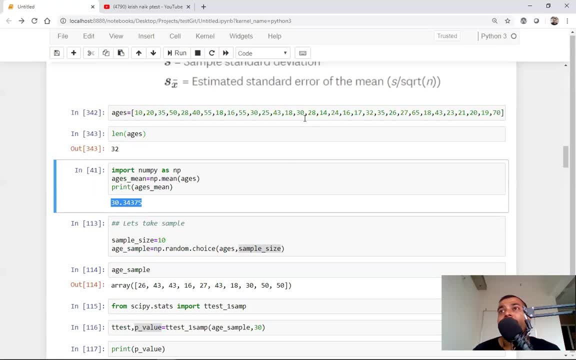 That is what I'm going to do Now from this population. what I have to do now is that take a sample of values Now I'm going to consider that out of this 32, I'm going to take a sample size of 10, okay. 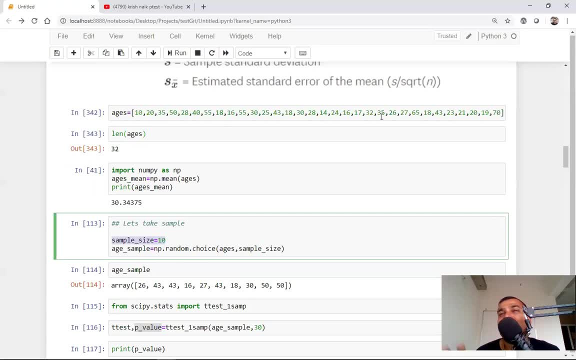 And inside this particular sample, I'm going to pick up this 10 ages randomly, okay, randomly. And inside this particular sample, I'm going to pick up this 10 ages randomly, okay, And inside this particular sample, I'm going to pick up this 10 ages randomly, okay. 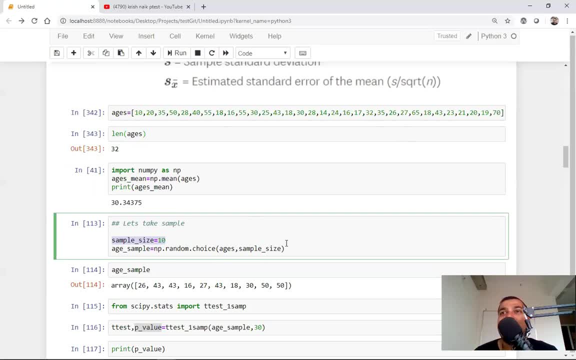 It will not be in some specific order, but I'll just be picking up randomly. For that I can use nprandomchoice, okay, And I'm giving the ages value, which is in the form of list, And this is my sample size, which is my sample number. 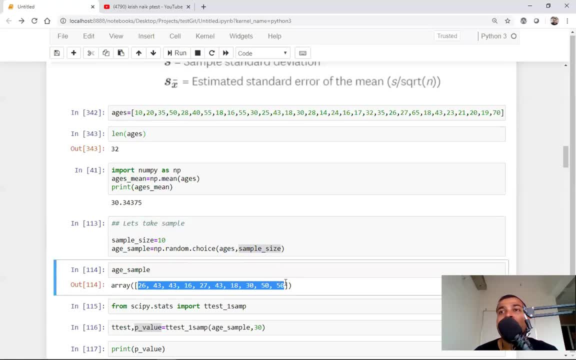 Now, if I go and see my age sample, I'm having all these particular values. Now, when I have this particular values, can I come to a conclusion that my sample mean and population mean are having a difference or not? okay, So for that, what I'll do is that, guys, I will just go in. 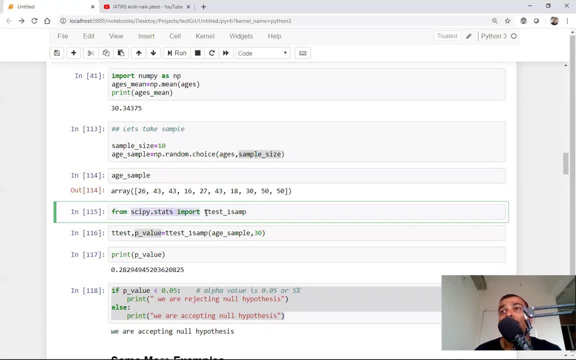 I'm going to import a library which is from skypie Feeling, which is from skypiestats. import ttest__1sample. okay. Now, this particular function is basically used whenever you want to perform one sample T test. okay. 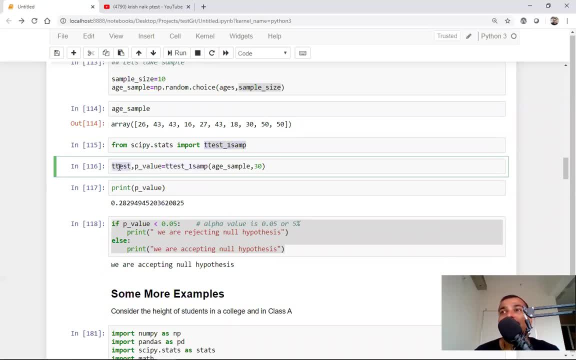 Now, this particular function will be gving you two values: One is the statistic T test value and one is the P value. The most important value for us is basically the P value. So, for that, what I'm going to do is that I'm going to use this t test. 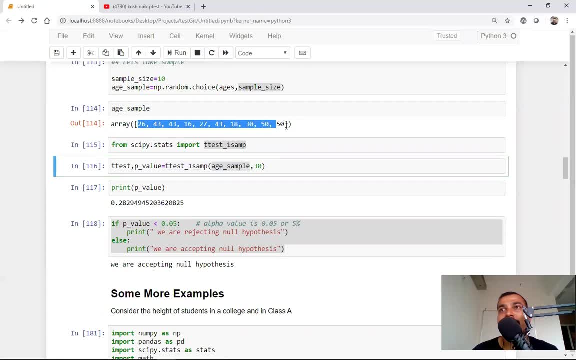 The first one, I have to give my age sample, which is all this, my this particular a sample, and then i am telling to compute whether this a sample is based on my population mean. suppose i say that my population mean is 30. okay, so if i want to compare this a. 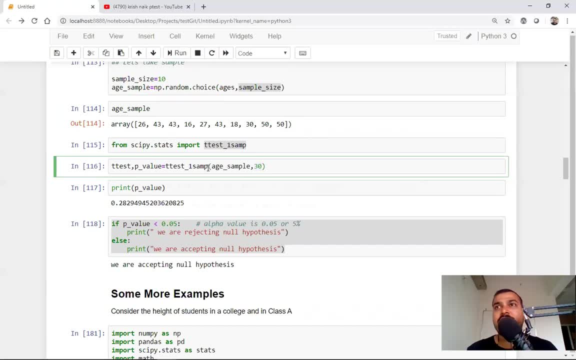 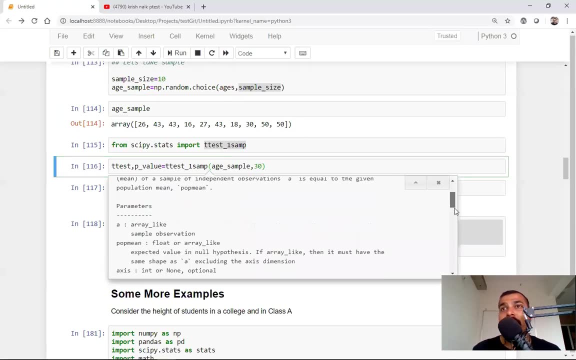 sample: is it b? you can just see. you can press shift tab over here and it says the calculator t test for the mean of one group of scores. okay, now if i go down and show you what is the meaning of, or the second parameter, that is pop mean. just understand over here. so pop mean is nothing but. 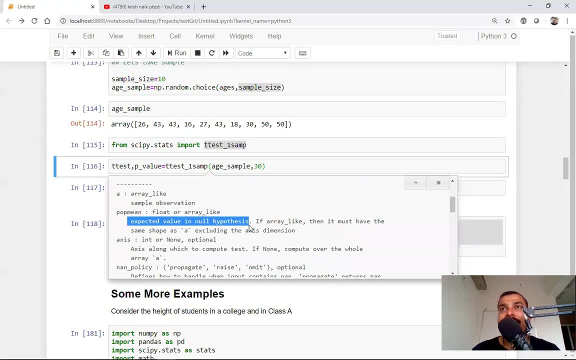 expected value in null hypothesis. so i am saying that, and my null hypothesis basically says that whether this value is going to be 30, which is which is which i am considering as my population mean- or whether it is not 30, okay, so if it is 30, what will happen is that we we say that there is 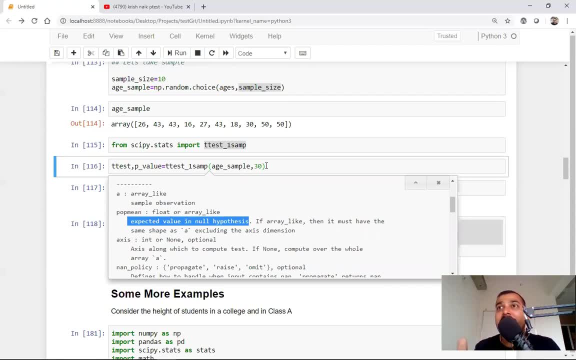 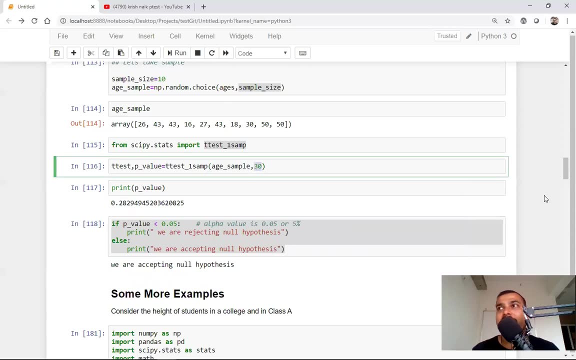 no difference. right, there is no difference. so i consider that that is a null hypothesis. in my alternate hypothesis there is a difference. how did i come up with this? particular values, guys, i've just taken randomly, considering my population, mean over here as 30.34. okay, so here i've taken it. 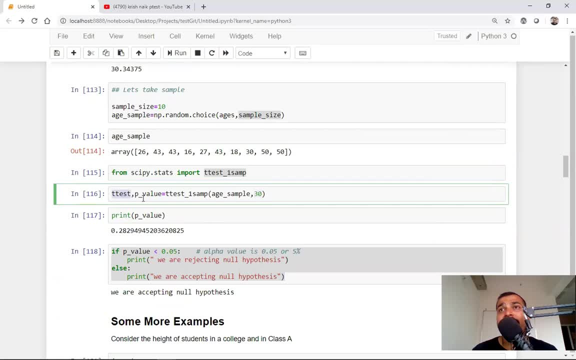 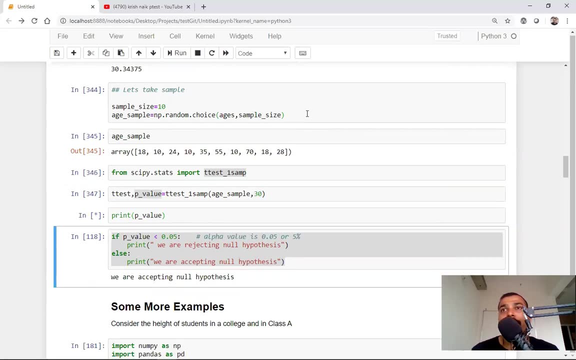 as 30. now, when i do this, you'll be getting two values. when it t tested on p value. if i go and print my p value here, okay, let's just let me take it once again. so here it is. my p value says 0.74. 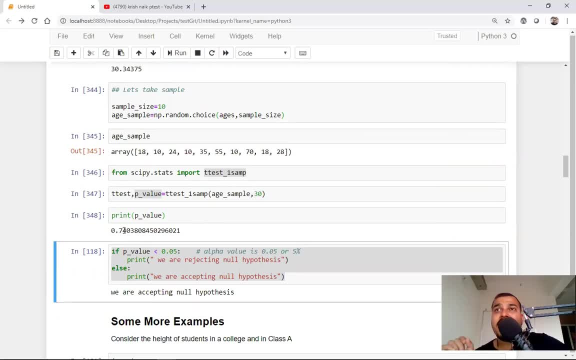 now this p value. we should say a condition, saying that again, guys, if my p value is less than 0.05, we are rejecting the null hypothesis. that basically means there is definitely a difference between the population mean and the sample based on this particular sample that we have actually. 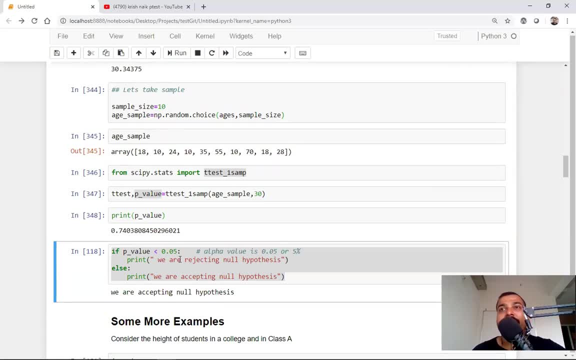 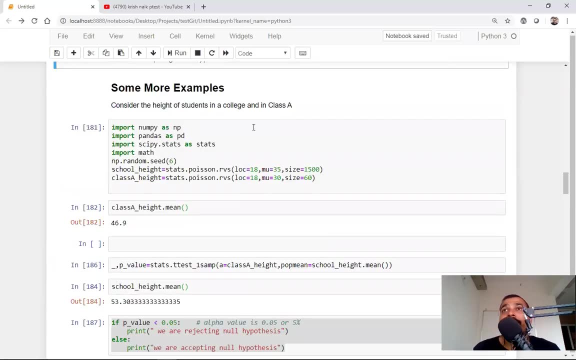 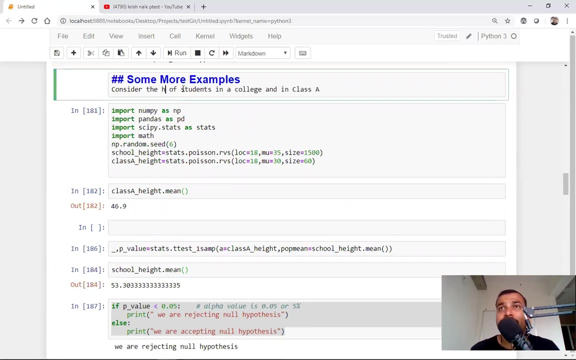 taken. so we are going to reject the null hypothesis in this particular case. now, this was just a simple example. okay, let me just consider some more complex examples. okay, over here i'm just going to consider: uh, suppose i let me just consider the age of our students in college. a okay, in. 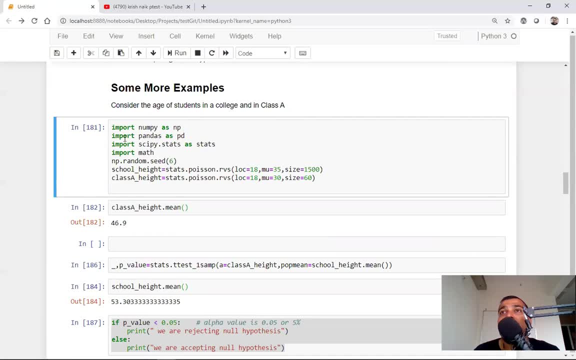 a college in class. now here i'm going to import numpy, panda, skypie, dot, stats and maths. okay, first of all, let me consider that in school i have more than 1500 people. okay, uh, in my school i have more than 1500 people, somewhere around 1500 people. so i'm going to consider a poison. 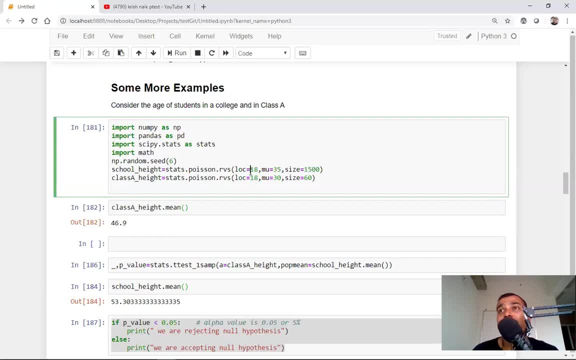 distribution saying that my age in that university or college starts from 18. okay, and this will basically be my mean 35. that basically means all my ages that are randomly getting selected will have a mean of 35. okay, it'll just be like a distribution or this: loc. 18 is basically. 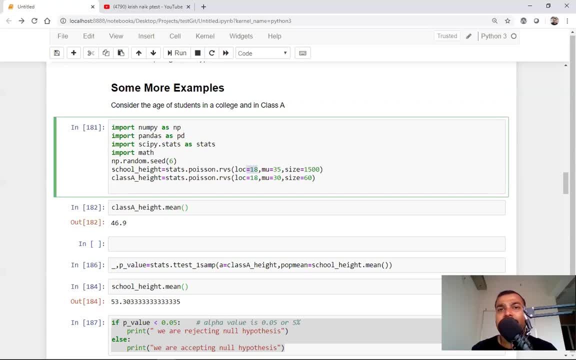 the most left value. okay, it looks something like this. i'll just draw it for you. so it will look something like this. so suppose this is my distribution. the mean will be 35, the leftmost value will be 18. okay, and based on this, the distribution will get selected for. 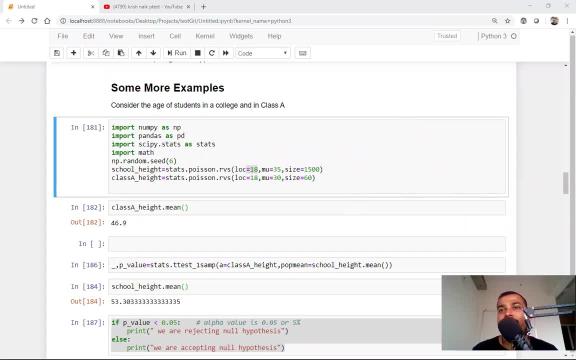 the school heights. okay, sorry, it should not be school heights. instead, i'll be taking this as ages. define it as ages, okay, and similarly class a underscore ages. i can also take height, not a problem. now, this is with respect to my school ages. okay, now, similarly, what i'll do for a specific 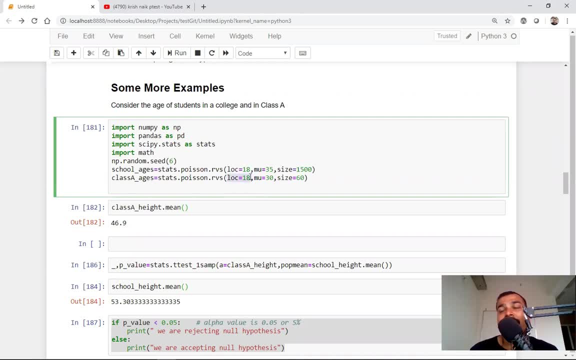 class. i'll say that. okay again, my left label. i'm initializing some values with respect to ages from 18, where the mean is 30 and i'm taking a sample size of 60 out of this 1500. okay, so here i'm executing it. if you want to really see what is your class, a underscore ages. here is my mean, okay. 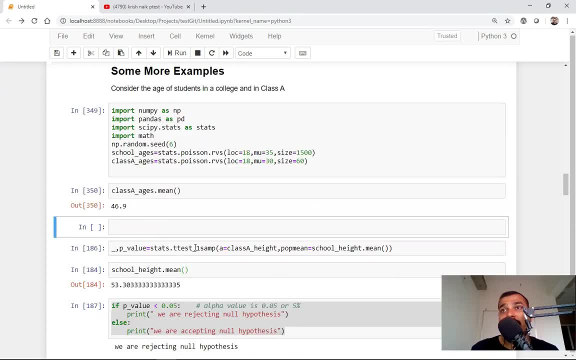 now what i'll do is that i can again use a test, one sample, to consider that whether this sample is different. the mean of this sample is different, that of a school underscore ages. so for this, what i'm going to do is i'm going to copy this again. i'm going to use t test underscore. 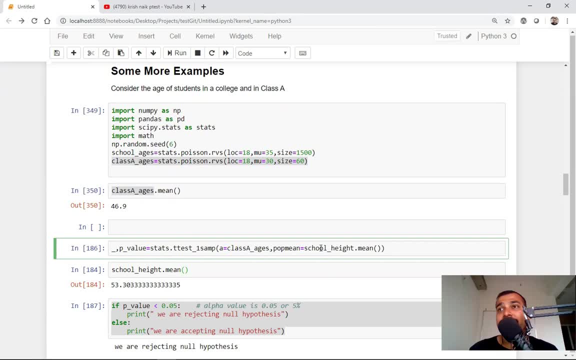 one sample and i'm going to paste it over here. and remember guys, this time my popup is going to be the same as before, so i'm going to paste it over here and i'm going to take the population mean. the second parameter which i'm going to take will basically be my 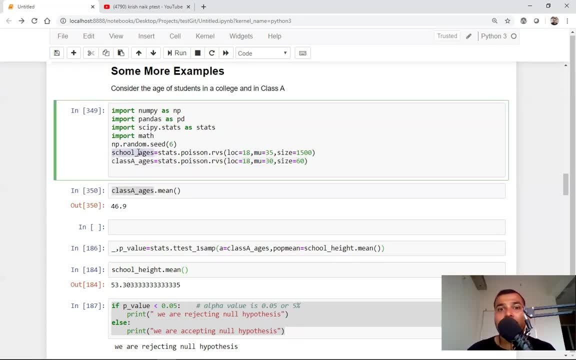 school height, uh, school ages, uh mean, okay, i've just written school height, so don't don't worry about that confusion again. this whole, uh, this jupyter notebook will be given to you. now. i've got executed this guys. remember again the first parameter: i have to give my sample ages. my second: 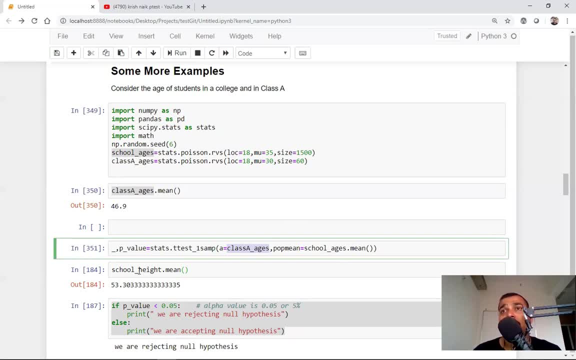 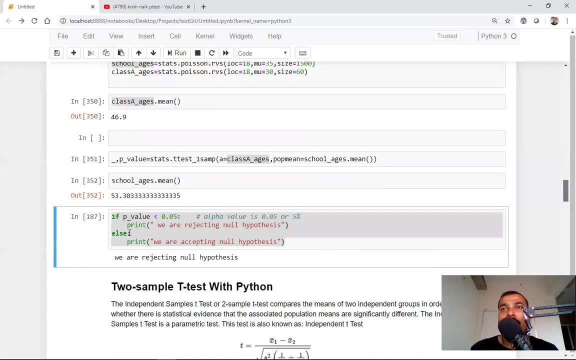 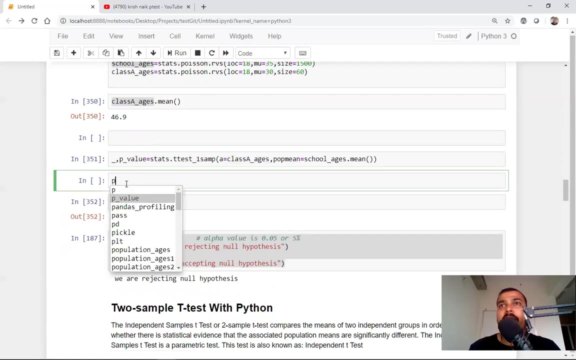 parameter should be the mean of my population. okay, now, if i go and compute first of all my school ages dot mean this is somewhere around 53.3. okay, now, again here i'll be getting my p value from this particular test. let's see the p value. okay, p value. and the p value is very, very less than 0.05. so if i execute, 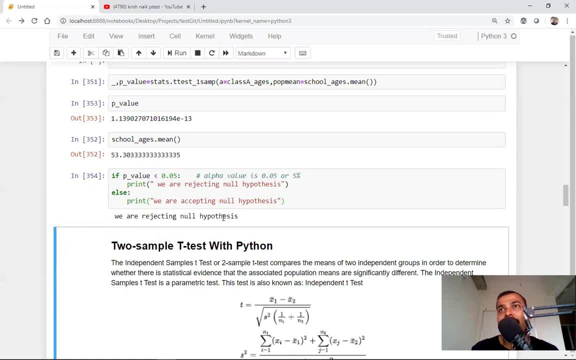 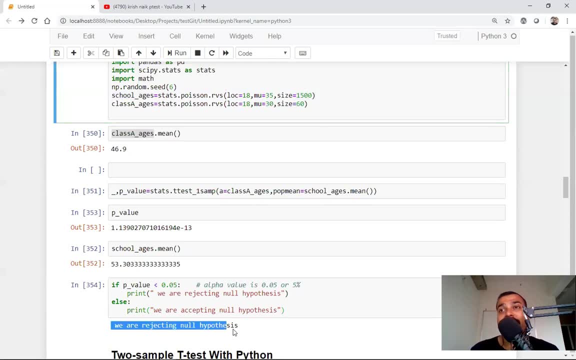 this particular statement. we are basically rejecting the null hypothesis. the reason is that the p value is less than 0.05. now, what does this mean? okay, what does this p value? and what does this basically say? we are rejecting the null hypothesis. understand that, guys? the p value is. 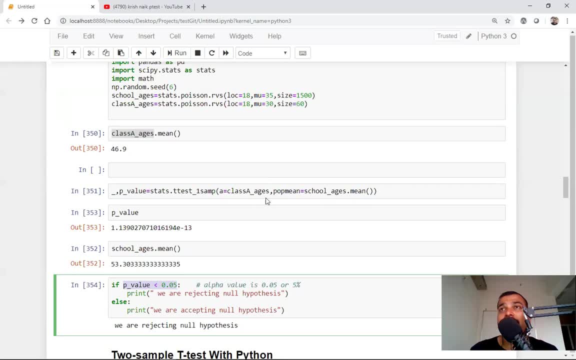 0.05. okay, now, when the p value is less than 0.05, that basically means we are rejecting the null hypothesis. the null hypothesis says that, uh, there is no difference in the mean of the age, whereas the alternative hypothesis says that there is a difference in the age right age. uh, difference in. 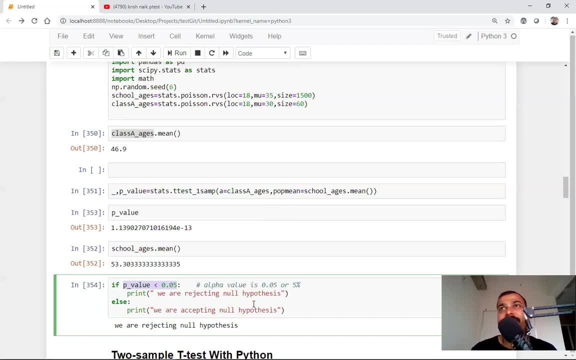 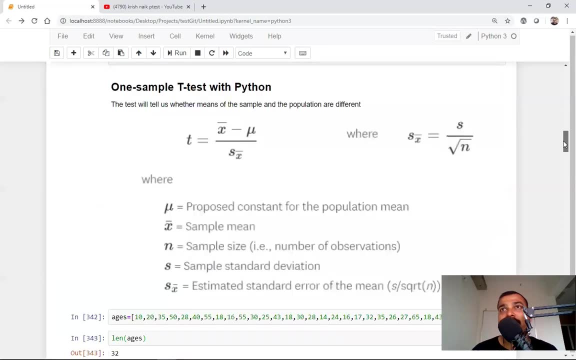 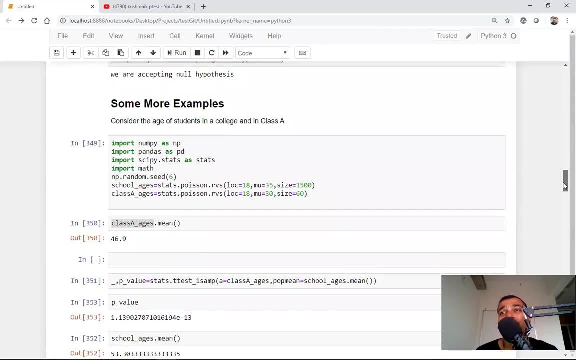 the mean of the age. now, in this particular case, there is definitely a difference, uh, in the age mean. so because of that, we have got the p value less than 0.05. so this was one example, two examples. uh, you, you are able to understand it. just go through this, you'll be able to understand more. 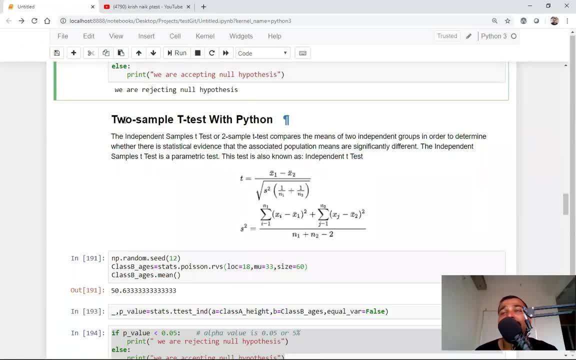 quickly. okay, now let me just consider another example, the second type of t test that is called as two sample t test. now the formula is this one guys, you need not remember the formula because you have libraries- the independent sample t test or two sample t test compares the two mean of two. 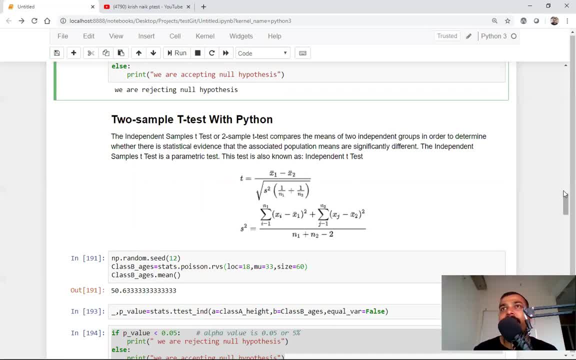 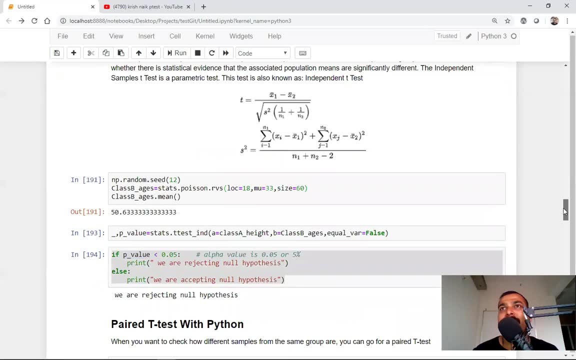 independent groups. now, initially, in all the above techniques that we did, we were actually trying to see in one group- right, you are taking a sample from the same group and you are taking a sample from the population. we are trying to see the mean over there. but in this particular case we have two. 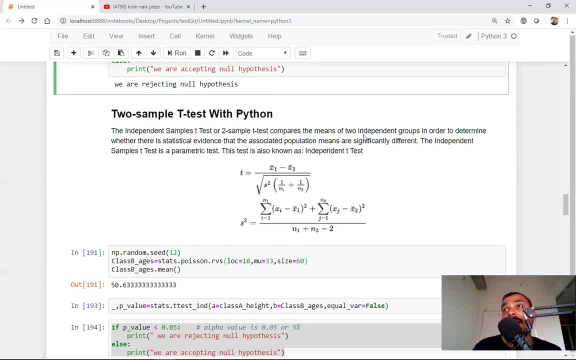 independent groups. now what we need to do is that we need to compare the means of the two independent group in order to determine whether there is a statistical evidence, that is, that the associated population means are significantly different. now here we are going to take the whole two groups. 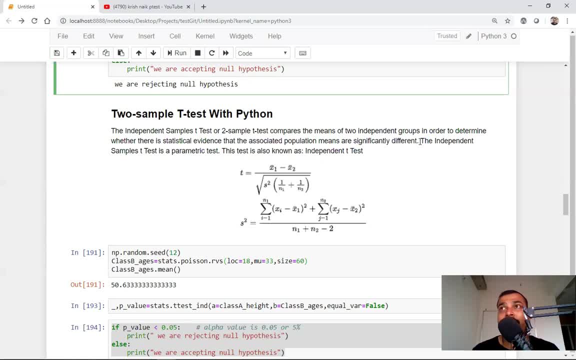 and then we'll try to apply a two sample t test with python and then we'll try to find out whether there is some statistical difference or not. if there is a statistical difference, that will be my alternate hypothesis. my null hypothesis will be that there is no statistical difference. okay, now what i'm doing. 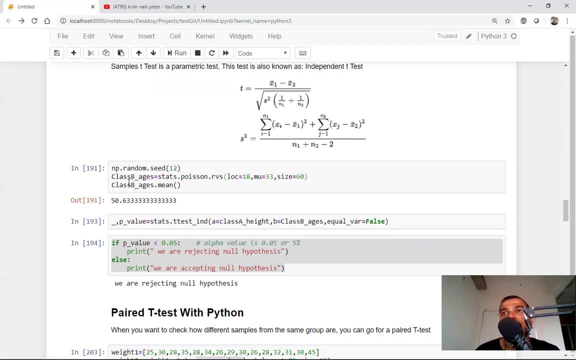 over here now in one of the class a ages i have initialized in the top. now similarly i'll initialize my another, class b. suppose there is another class there also. i'm going to take some ages and here again i'm using this poison distribution where my leftmost side label is starting from 18 h, the mean. 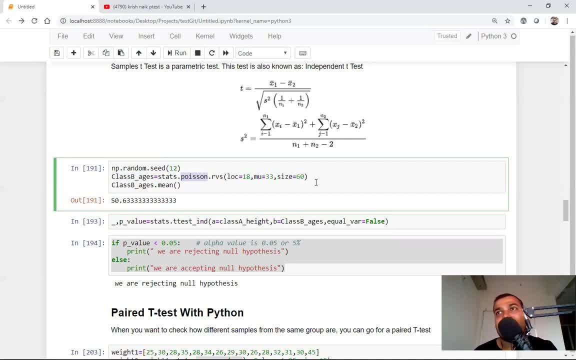 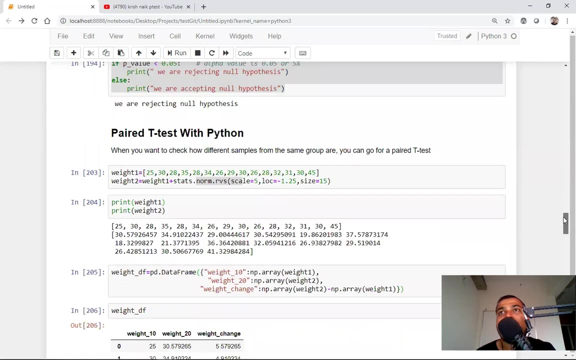 is 33, and again, here i'm taking the size of 60, okay, and if i go and compute this particular mean i'm getting somewhere around 50.63. now understand, guys. in the previous example we use something called as t test underscore one step here. our function name that we'll be using in this scenario in two sample t test, is something: 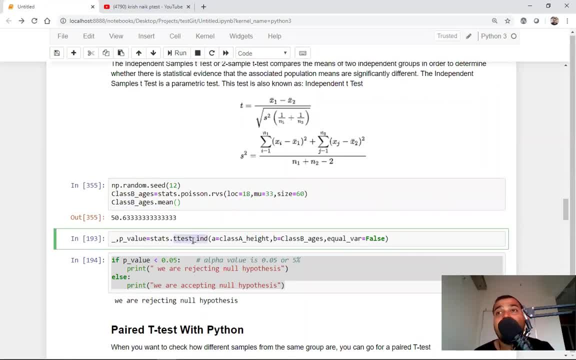 called as t test underscore int. okay, and here you will be requiring. the first parameter will be nothing but the a value. a value basically means one group, b value basically means another group. so here i'm specifying my a and b value, then i will just go and compute. 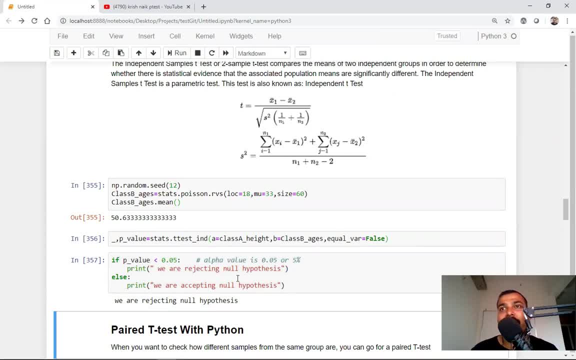 and if my p value is less than 0.05, we are rejecting the null hypothesis. in this case also, we have got the p value less than 0.05. that basically means there is some significant difference between the population mean of this particular two group, and this is how it is done. 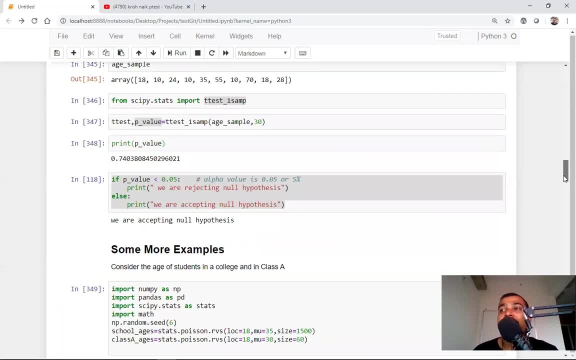 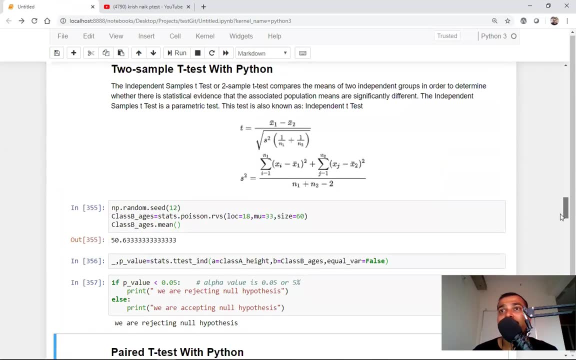 this is applied to the whole population. in the previous example, if i had a population, i'm considering some sample and then i am applying this particular test. so this was the basic difference between one sample and two sample test with python. uh, there is also a third technique which is called. 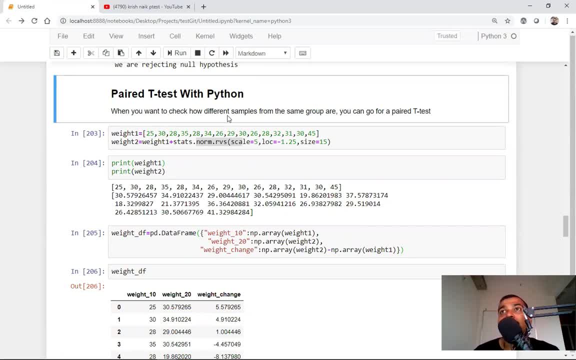 the p-test. okay, now, when do we use this? when you want to check how different sample from the same group are, you can go for pair t test. now, what does this basically mean? uh, again, i'm reading it for you guys. when you want to check how different samples from the same group are, now consider this particular. 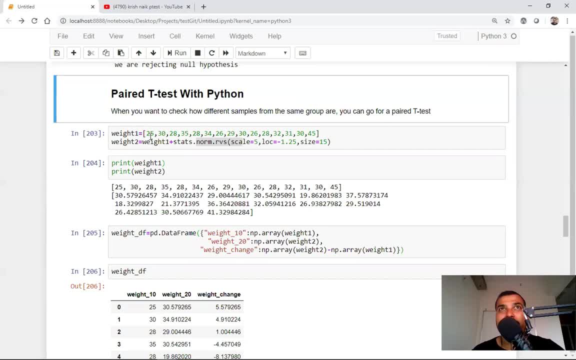 example, i had some weights of the student over here or some weights of the school kids you know, and school kids, if you know that, if they are, if the age is somewhere around 5 to 15, the ages, the, the basically ranging between these values, right, 25, 30, 28, 28, 34, 26. so small kids have just taken an. 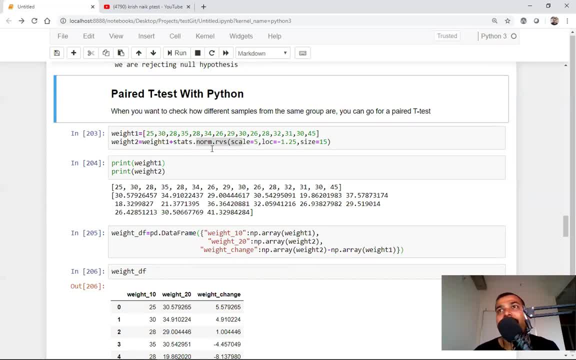 example. now consider that after some years the weight have actually increased. so what i have done is that i have again created another list over here. my weight: 2.. uh, this has added some normal distribution value. considering my scale as 5 location, as minus 1.25 size, is equal to 15.. so 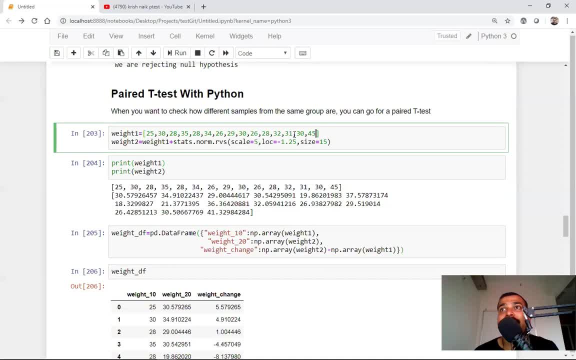 15 values. i have added. why 15 values? because this, this, the length of these values are 15.. okay, so i am append, i am adding some more weight on top of these particular values. i am considering that after some years, the age, the weight of those people, of those child right, will be increasing. so, based on 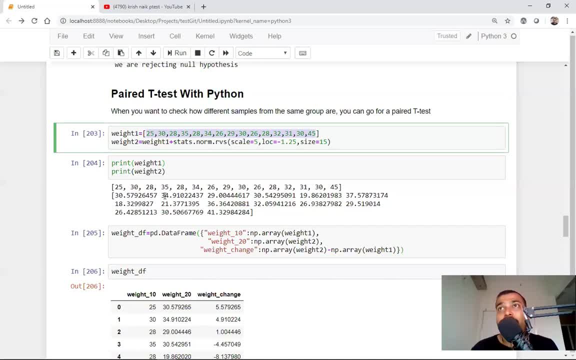 that i have to print it with weight 1 and weight 2.. now we need to go and see that whether, whether whether weight 1 or weight 2 have a statistical difference or not, or how different these particular samples are right. so my alternate hypothesis will say that there is no such- uh sorry, there is a statistical difference. 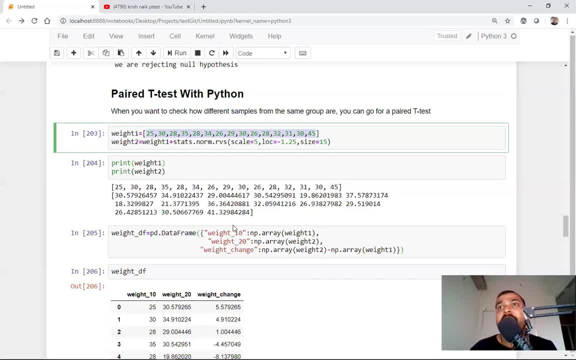 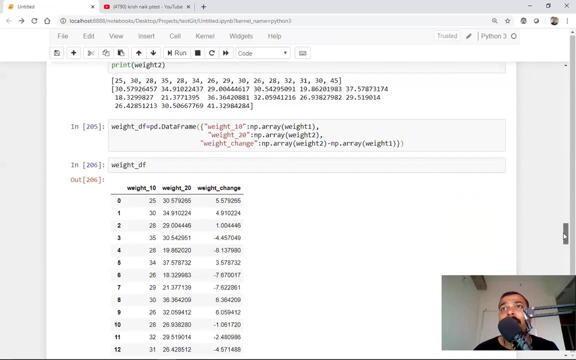 whereas my null hypothesis will say that there is no such statistical difference. now, if i want to compute in this particular way, we basically use a paid t-test with python, because we just have same group, okay, only the sample values has been changed right now, in this particular case, i'm going to take this, okay, and here you can see that i'm combining. 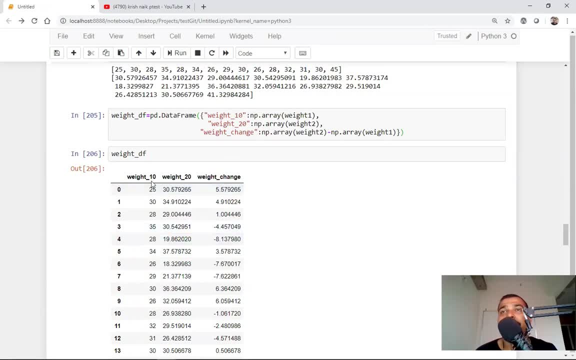 this all into a data frame. and this is my weight change that has happened from weight this, two and this. okay, uh, weight this to this, uh, this changes have been happened. you can see that i've actually created this data thing. now what i'm going to do is that for that, for this specific reason, i have 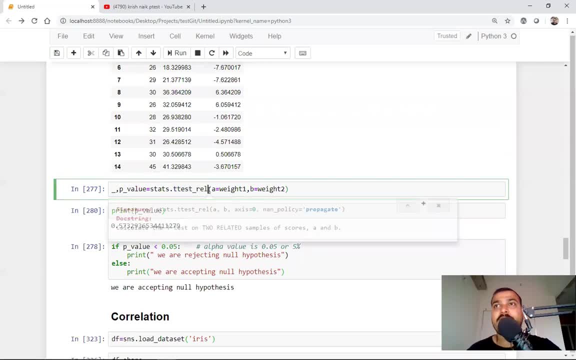 to use t test underscore real r, e, l. if i press shift tab, you'll be able to see calculate a t test on two related samples of scores, a and b. okay, now here the value i have to give: the previous weight and the recent weight. now, when this two is compared, you know we'll be able to get this. 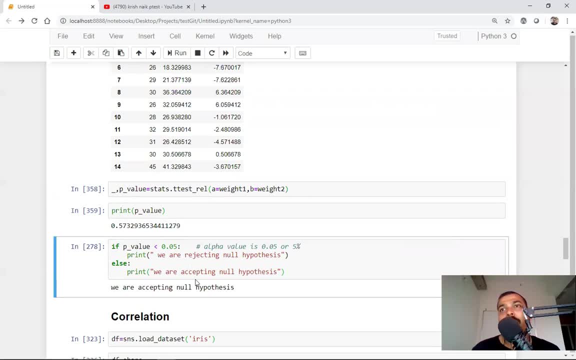 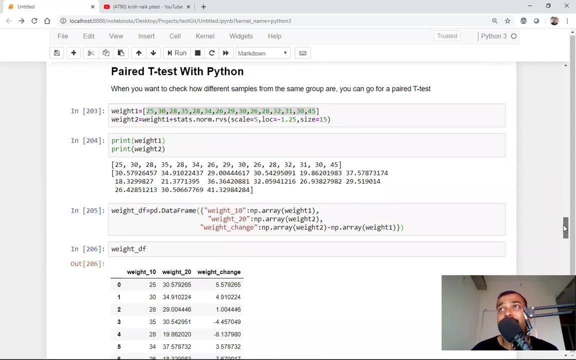 p value. again, if this p value is less than 0.05, we are rejecting the null hypothesis. in this case, we have to accept the null hypothesis because the p value is greater than 0.57. right, and here you can see that. uh, this basically says that there is no such maximum difference between these particular 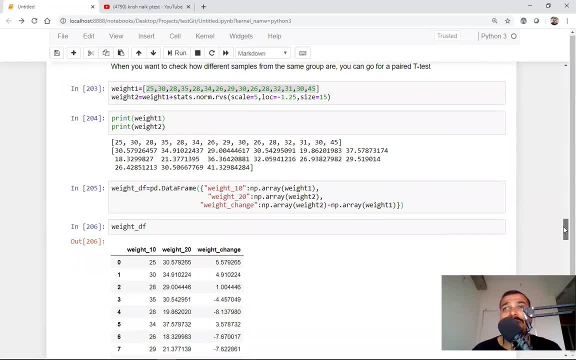 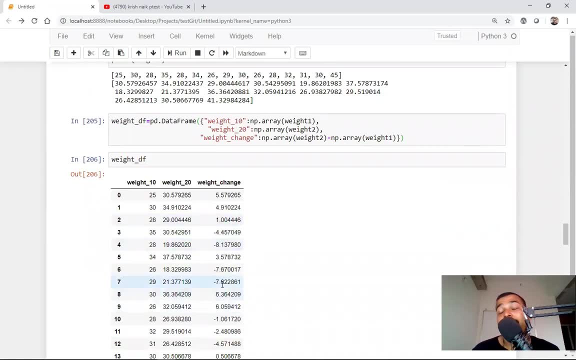 groups right, and then you can see over here that the values just increase a little bit. so because of that you are, you can see the difference. also minus values have also been increased. i mean there is also deduction some amount of values because it has been randomly initialized here. uh, based on this normal. 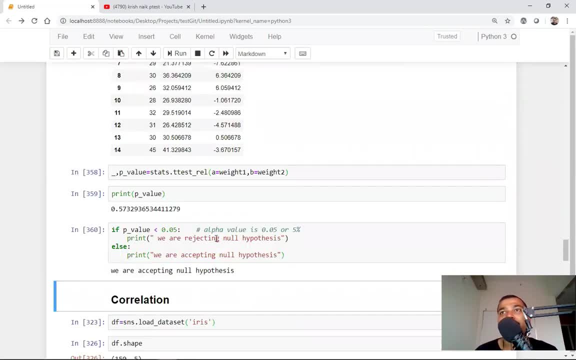 distribution that we have used. now, in this case we are not rejecting the null hypothesis because the type of values that we have got in these two fields looks almost same, so there is not much that difference when compared to the- uh- initial weights that we actually had. so this was the three kinds. 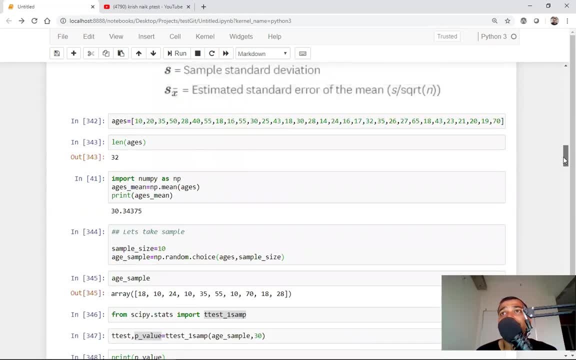 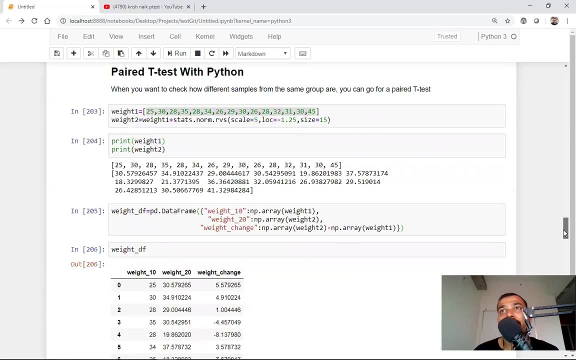 of t test. again. just try to do it, guys. uh, if you have any queries, please do let me know in the comment section. one sample t test with python, uh. two sample t test with python and pair t test with python. now one more example that i want to give is: 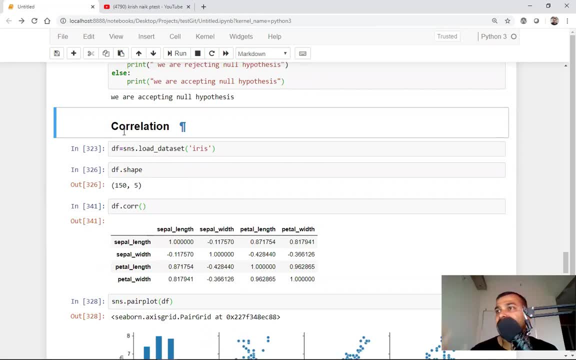 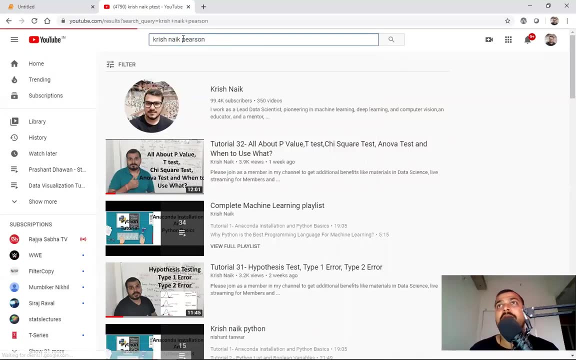 something called as correlation. now, correlation guys. if you have not seen my pearson correlation video, just go and search krishnaik pearson. okay, just search it like that. uh, what is pearson correlation coefficient? what is the difference between correlation? covariance is given over here. 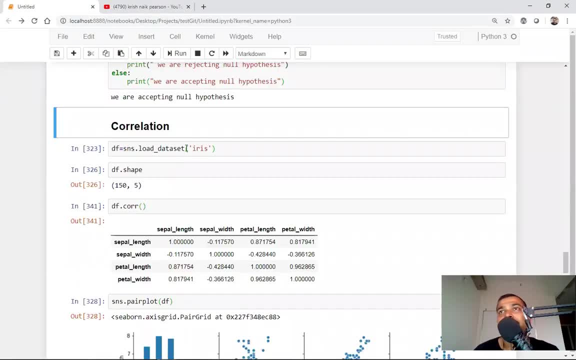 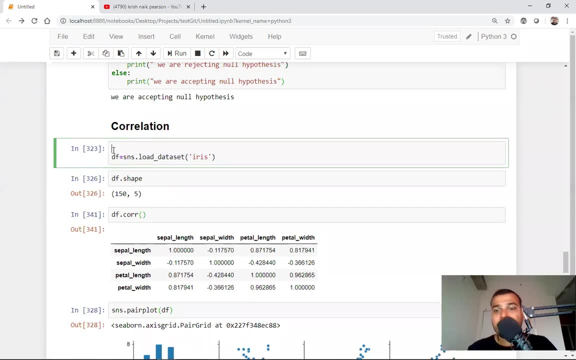 explained pretty much clearly. now what you have to do is that here i'm going to consider some irish data set. so here is my irish data set that i've actually had the initial data set. i've concerned uh taken instead. what you can also do is that import c bonus, c sns. okay, so snsload. 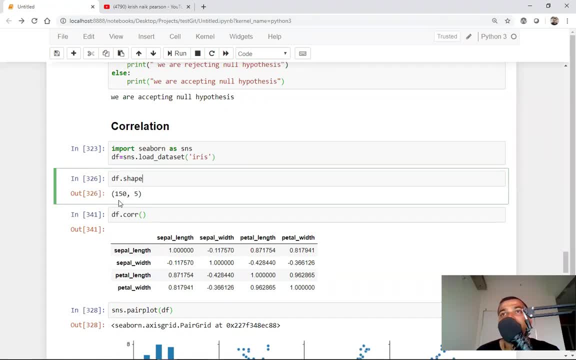 underscore data set: iris. okay, and this is my iris data set shape. now, when i'm doing the correlation, always remember, guys, according to pierson correlation, your values will be ranging between minus one to plus one. okay, now, if you see this particular condition over here, my sepal length: 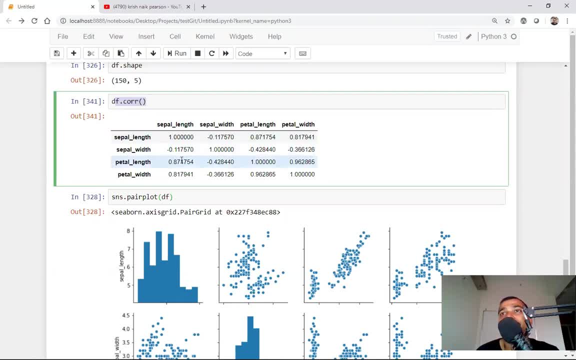 sepal width, petal length and petal width. wherever you see some maximum values. now, in this particular case you can see petal length and sepal length. they are highly correlated. somewhere around 87 percent if the value is nearer to zero. that basically means that it is not that much correlated. 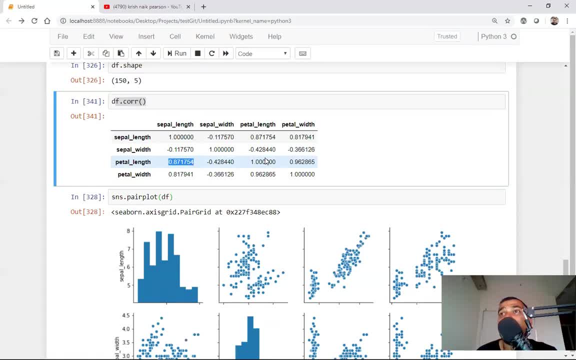 if the value is negation, like completely negative, one minus one, like that right or nearer to minus one, or like minus eight, seven, five, something like that, okay, at that time it is inversely correlated. now this particular value, you can see that 0.96 is very, very highly correlated. so based on that, 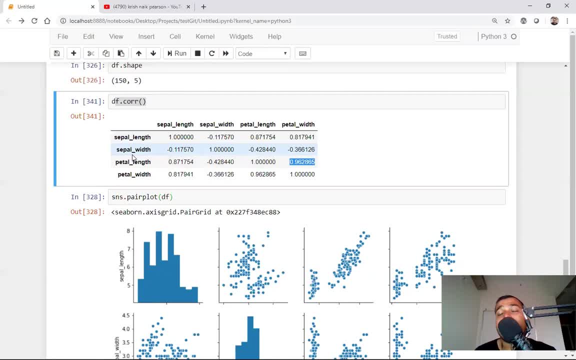 you can actually select what all parameters are important when considering the dependent features or independent features, right? so this correlation also gives you a whole lot of idea regarding that, and this is majorly used in feature selection also. there is one more example that i would like to give that this correlation values over here is 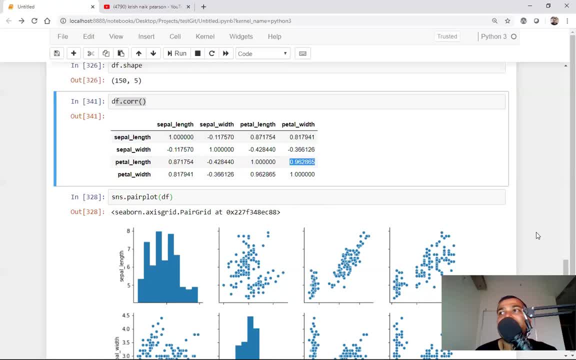 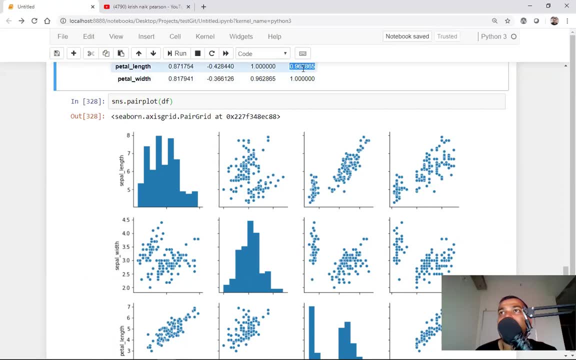 some numeric values or floating values, right? if you want to represent this in the form of graph, all you have to do is just write snspairplot. you'll be able to see the graph. now you can see this particular value, right, point nine six, two, eight six five. if i go to the graph and i'm going to 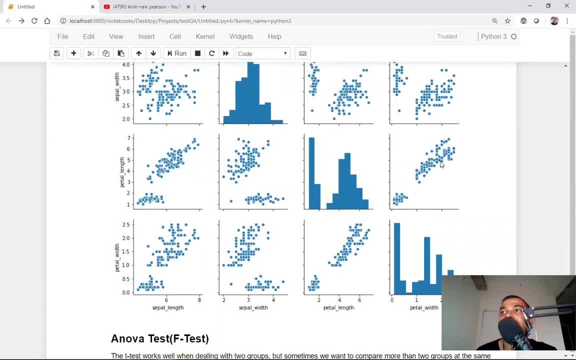 go over here, guys. this is that graph. you can see that how linearly it is correlated, right, because of this, this is having the maximum value. you know. it is having some linear representation with respect to your petal length and petal width, which is, you can see, in the right hand side. so, yes, this was all. 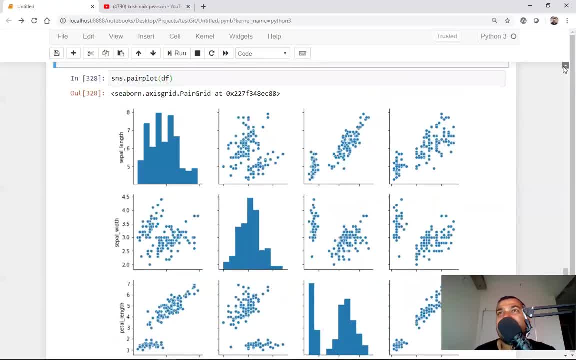 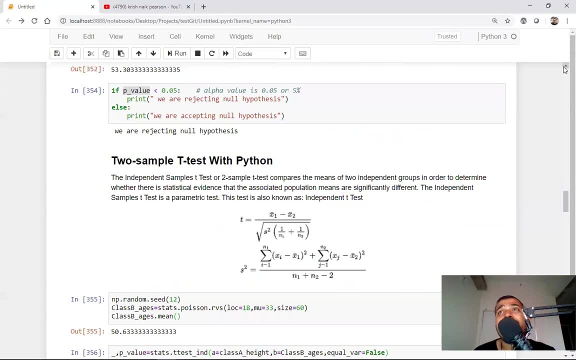 about this particular video. i hope you like it again. guys, there will be definitely some confusion regarding it and it is not that simple. you need to learn a lot, but understand that we we perform this steps in some of the steps that we perform in the next steps that we perform in the next steps.